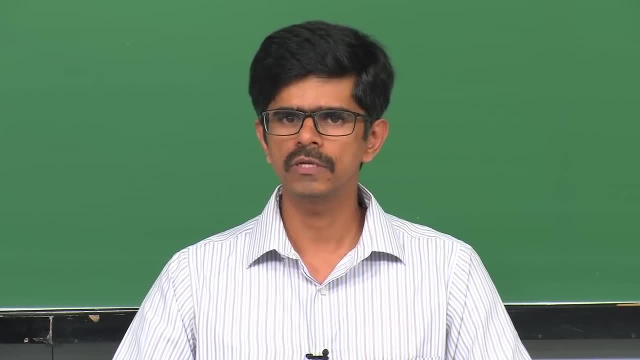 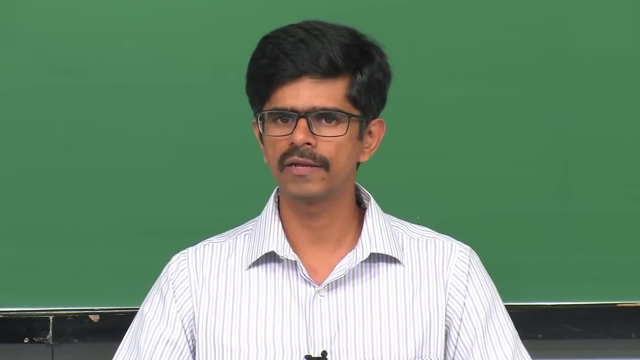 one day to do the job. Now the job is done much more quickly because the 10 men are working in parallel. So each man just needs to do one tenth of the entire job, and the entire job is just completed within a single day. So this very same concept. 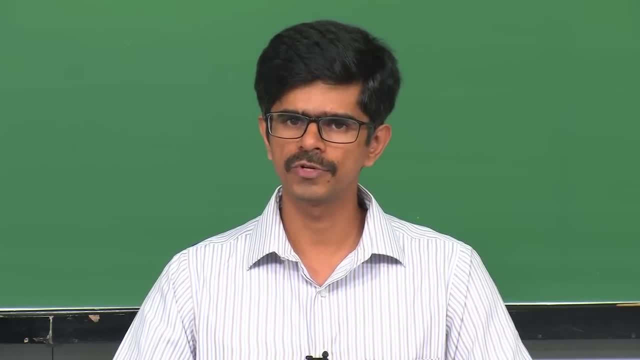 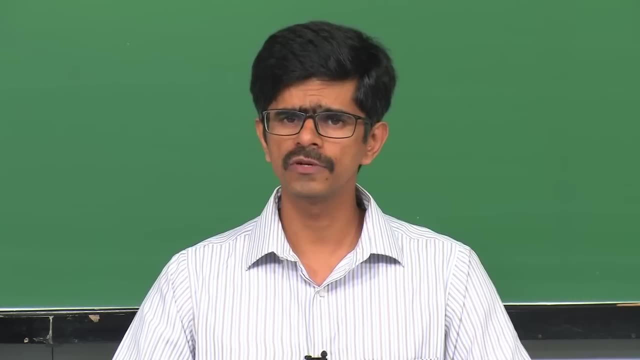 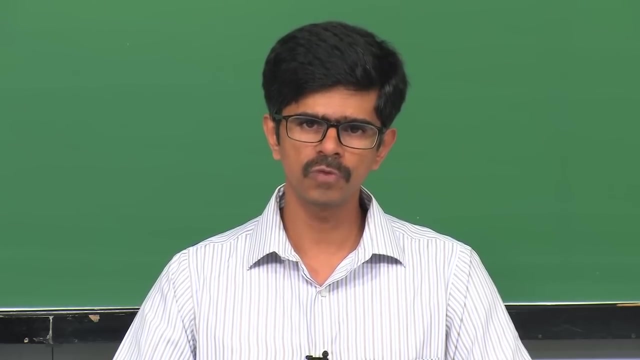 of parallelization is applied extensively in computer systems. Essentially, parallelization in computer systems are used quite often to improve performance of applications. So what is done is that if there is a large job to do, we will parallelize it in the system. 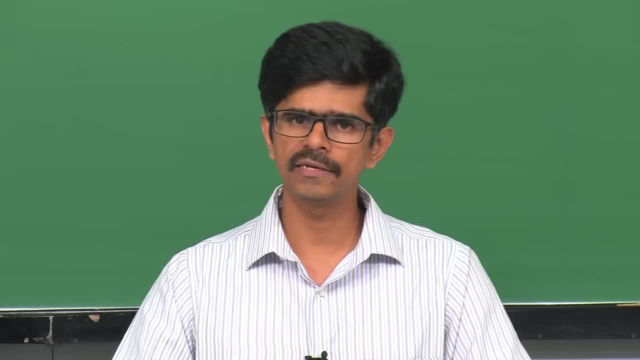 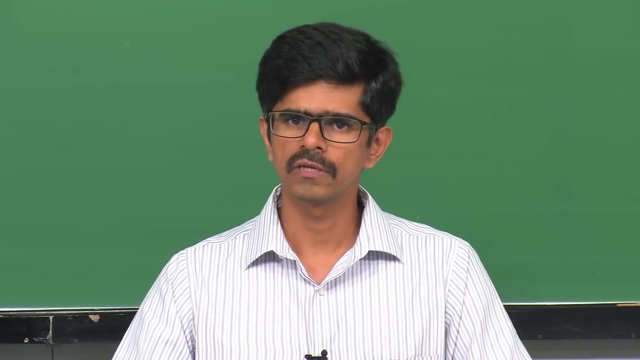 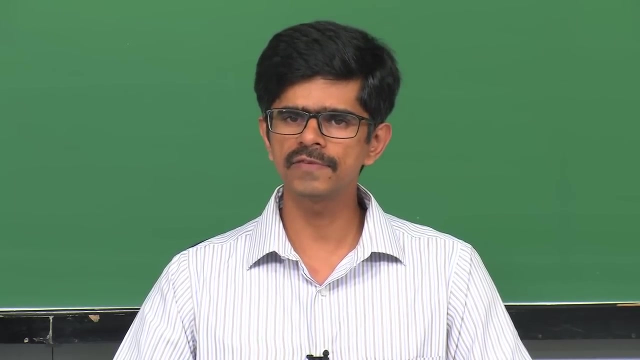 So that different computing entities- these are computing entities which are very small and do a small portion of the larger job, and these computing entities execute in parallel and altogether the job will complete much more quickly. So these days parallelization is extensively supported by several computer hardware In 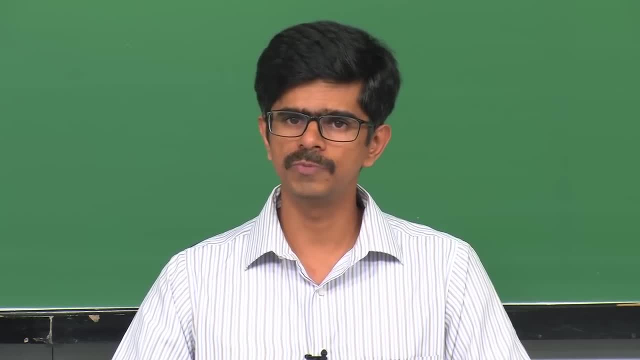 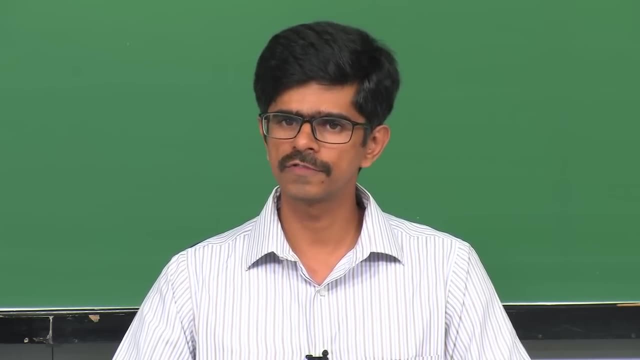 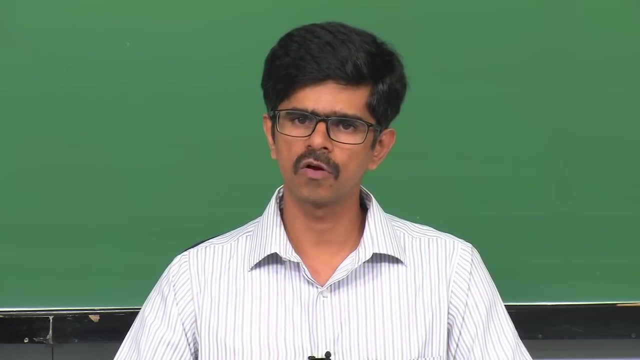 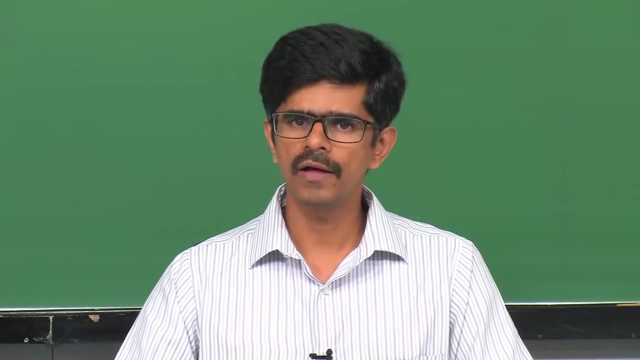 fact, there are some hardware that is present which are called GPUs, or graphics processing units, which are capable of performing thousands of tasks in parallel. So each of these tasks are a very small part of a larger job, but the fact that all these tasks are done in parallel will 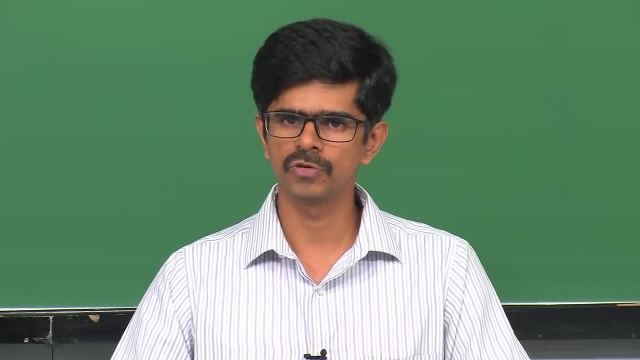 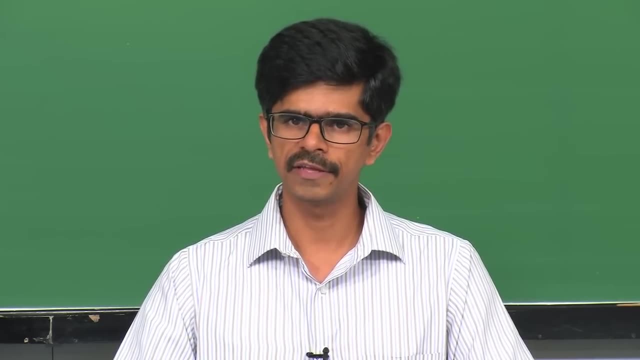 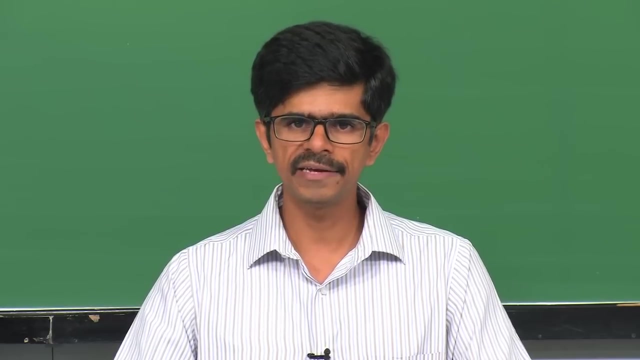 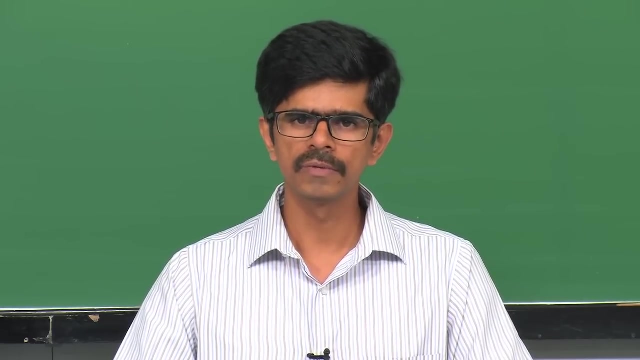 achieve a much more lesser time to complete the larger job. Now one construct when doing parallelization is threading or threads. Threads are essentially execution entity, very much like processes which we have studied in the previous videos. However, threads are extremely light weight processes and they are essentially used to make parallelization. 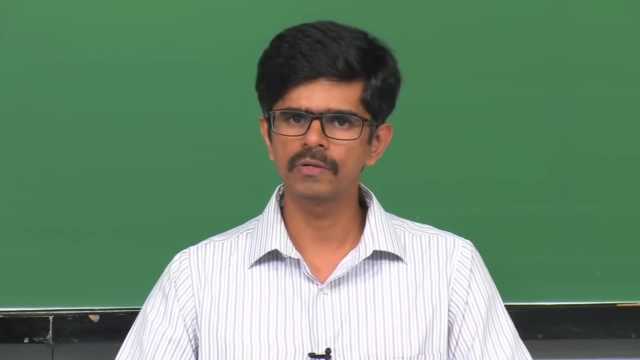 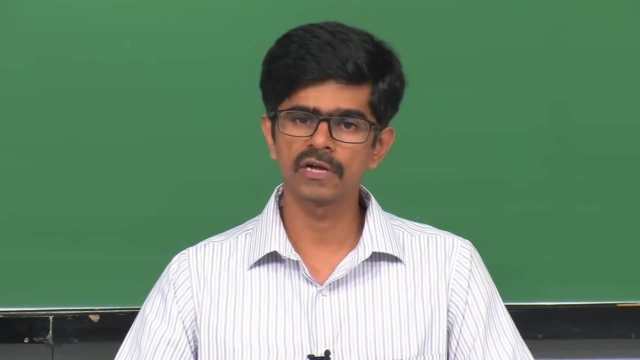 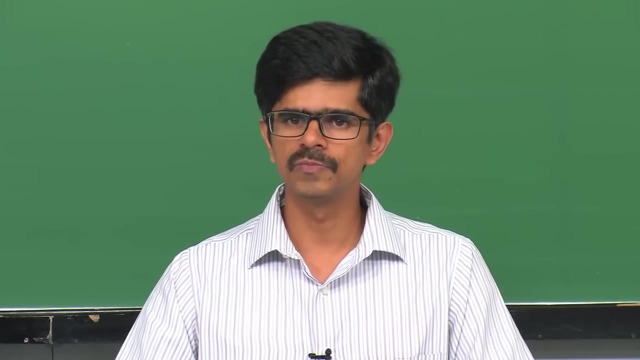 much more easy. So in this video we will look at parallelization. Thread is basically a process of creating a network of threads which is presented as a training network. The video will cover how the threads are created or destroyed, how it differs from processes and how different operating systems support threads in different 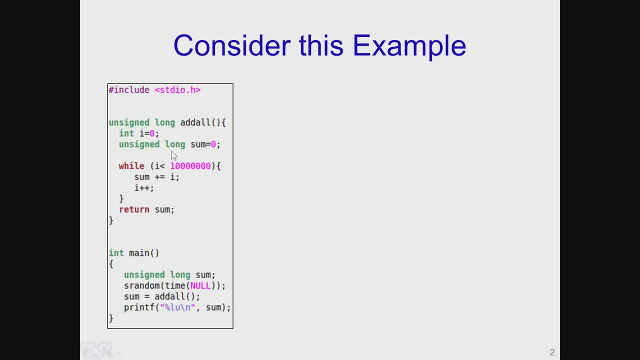 ways. So let us start this particular video with an example. So let us consider this particular program. Essentially, we have a function here called, which is invoked from main and returns unsigned long. So this function add all just sums up, or? 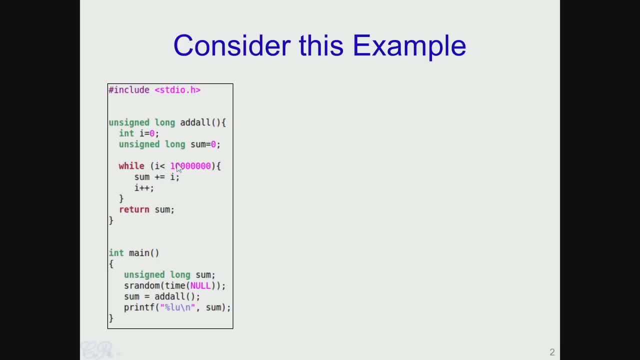 adds up the first 10 million positive integers and the sum is returned over here and printed in the main function. So obviously this particular program could be written in a much more different and much more easier way without having to iterate through every number from 0 to 10 million. However, for sake of understanding threads, let us go with this. 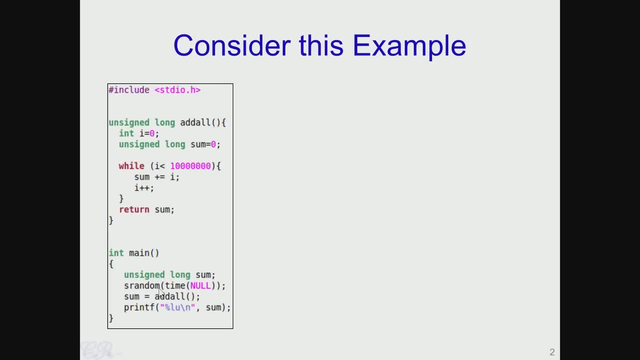 particular program. So what we have seen in the earlier videos is that when we, after we write this program, we use a compiler such as GCC which creates an executable, and then that executable is run to create a process. So we will eventually have a process which has its own memory space, and part of it may 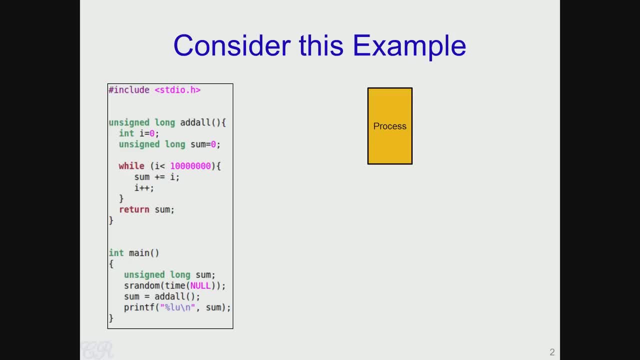 be in the RAM. and now let us see what would happen if this process is executed on a system with, say, 4 different processors. So what happens is that the scheduler in the operating system is going to pick up this process and assign it to one of these processors. So 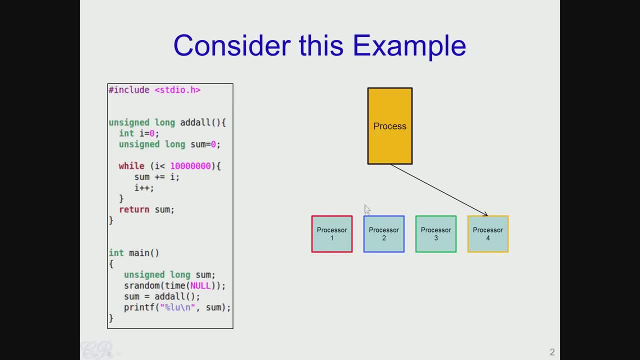 So always, once assigned, this process will be executed in one of these processors, and rarely this process may migrate to other processors. but let us not get concerned with that Now. what we observe here is that, even though we have 4 processors present in the system, 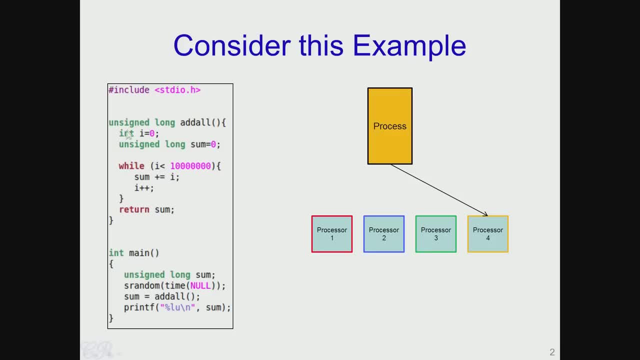 this entire program, which may take considerably long to execute on a system just runs on a single processor, leaving the other 3 processors idle or doing some other task. Thus the execution time of this entire program will be quite large, because this sum is found sequentially by iterating through all numbers. 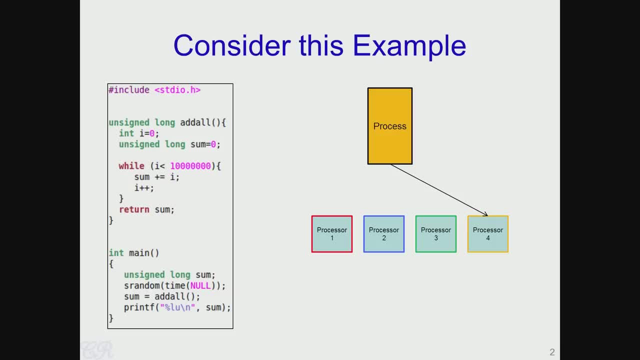 From 1 to 10 million in a sequential manner, as done in this particular while loop. So, given that we have a hardware like this with 4 processors, this is not a very good way or efficient way to write this particular program. So what can we do better to make this program parallelizable and make it to execute on all? 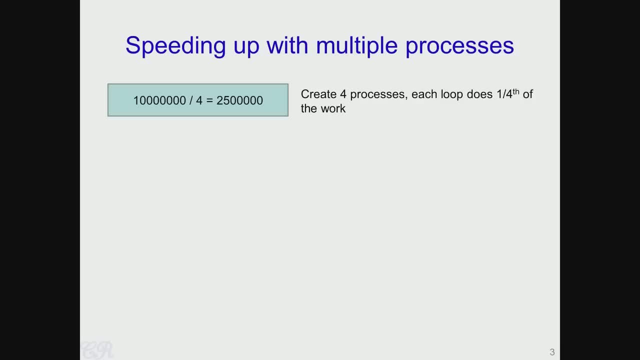 these 4 processors. So what we will do Is that we will take 10 million numbers and divide it by 4 to get 4 quarters of 2.5 million each. So then we would create 4 processes, and each process will loop through a quarter of these. 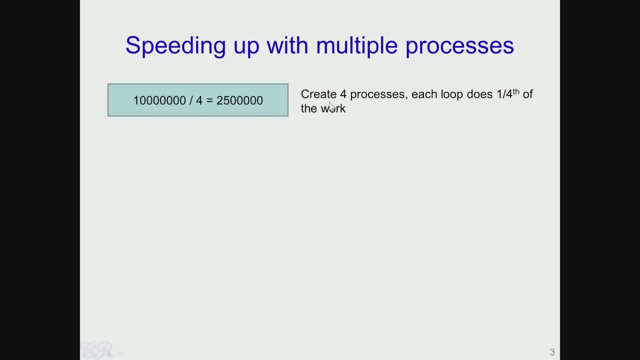 numbers. That means the first process would loop through numbers from 0 to 2.5 million and find the sum of Of all these numbers. the process 2 will find the sum of the numbers from 2.5 million to 5 million. process 3 would find the sum of numbers from 5 million to 7.5 million and. 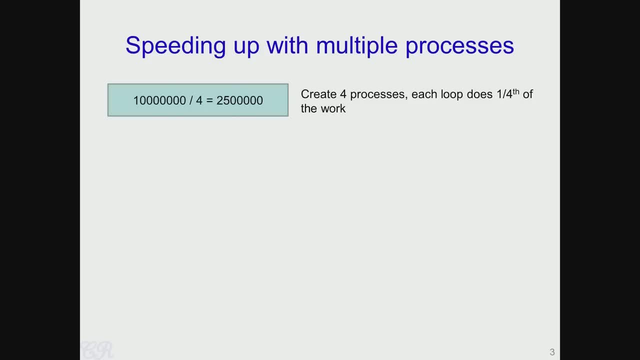 process 4 will find the sum of numbers from 7.5 million to 10 million. So if we are able to create 4 processes in such a way, then when we execute these 4 processes it will work. So that is it. 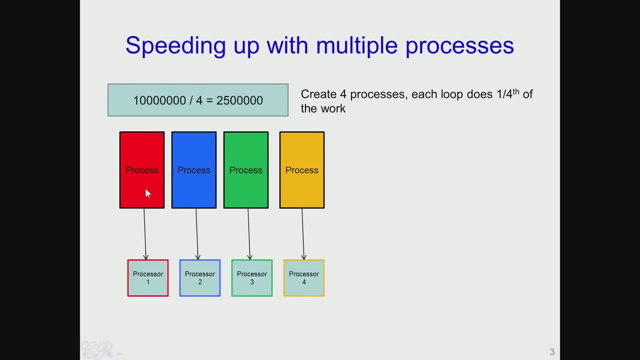 It will be something like this. So each of these 4 processes execute on a different processor in the system and each of these processes just do a smaller job of finding the sum of 2.5 million numbers instead of finding the sum of the entire range of 10 million numbers. 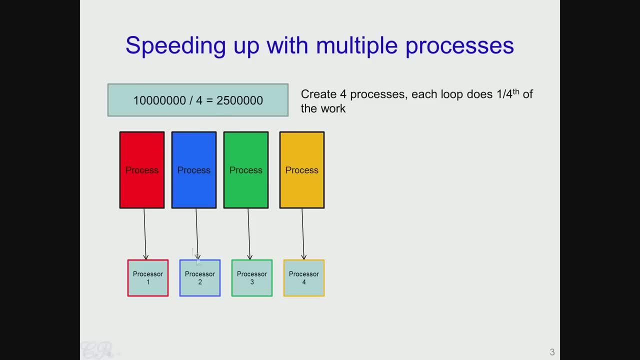 Further, since each process is scheduled in its own processor. therefore, we get parallelization, So we get parallelization. Thus, what one would expect is that the entire program of finding the sum of the 10 million numbers can be completed 4 times faster. 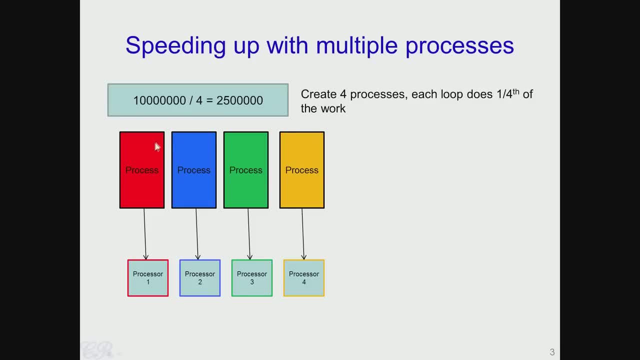 So this seems to solve our problem of parallelization and it will more effectively use the processes present in the system, And some of the properties that we have of this particular approach are as follows. So in order to create this particular 4 processes, we would require 4 fork system calls. 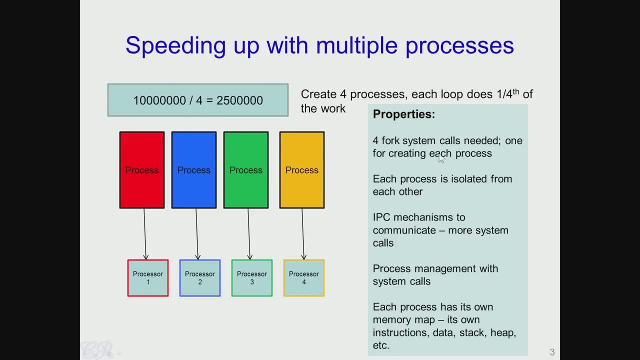 So each of the fork system calls that we invoke would create one of these processes. Further, what we notice- another property of this particular model of speeding up or exchanging numbers, So the fact that the 4 processes are achieving parallelization- is that each of these processes 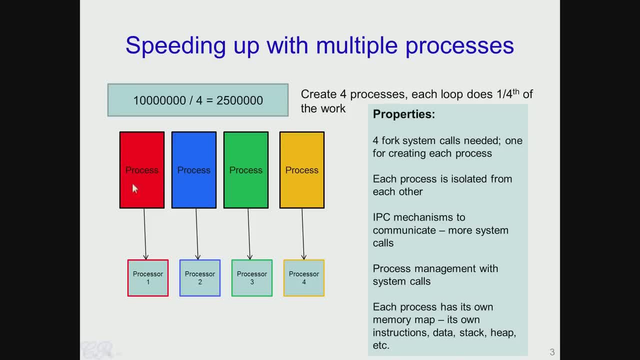 are isolated from each other. That is, each process has its own set of instructions, data heap and the stack, and these segments in this process are isolated from the other processes among these 4.. Next, due to this isolation, we require inter-process communication technology. 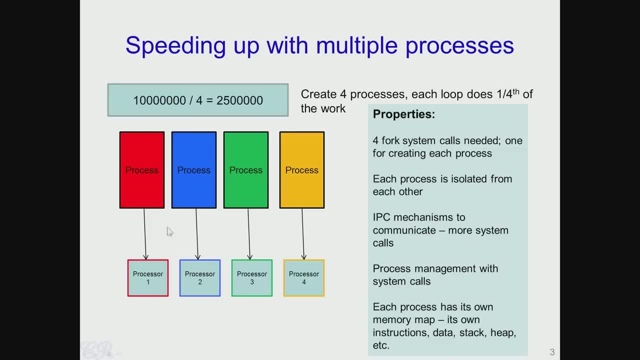 We call it IPC or IPC-based communication technology In order to communicate with one process with another. so we have seen that IPCs can be achieved in several ways. So one way is by having the send and received system calls and the operating system will. 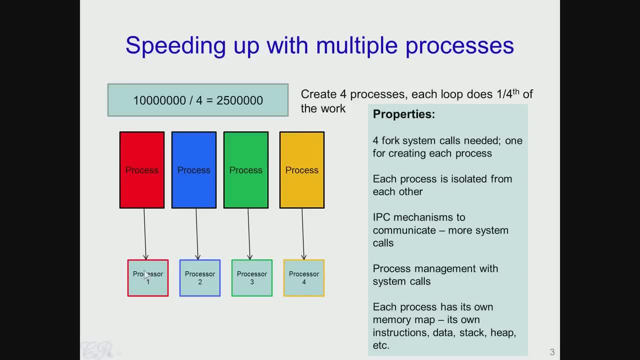 help in creating a channel through which IPCs are achievable. The other ways are by shared memories Next, or in which case a shared memory is created in one of these processes, again by use of system calls, and this shared memory is can then be used for IPC's between the processes. 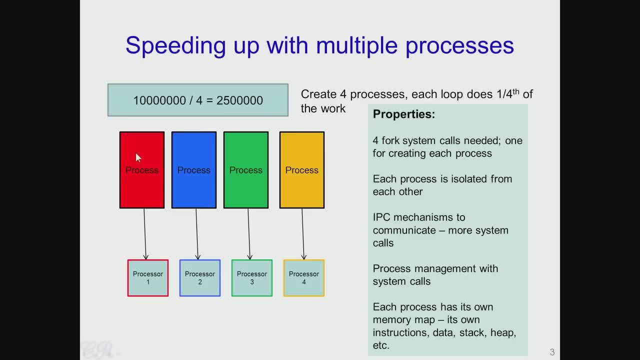 Further, since there are various stages in the process, such as the creation, destroying or file operations and so on. so all these process management activities are done through system calls. and also the last point, as we have mentioned, each process has its own isolated memory map comprising of instructions, data, stack and heap. 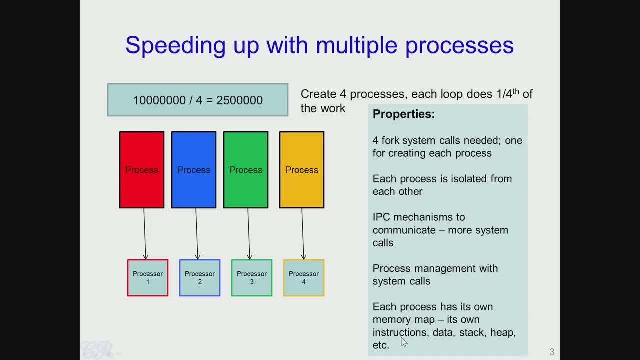 Now, what we notice among all this, from these properties, is that there are considerable amount of system calls involved in solving this problem in this particular way, that is, by having multiple processes to perform parallel, And, as we have seen in an earlier video, these system calls have considerable overheads. 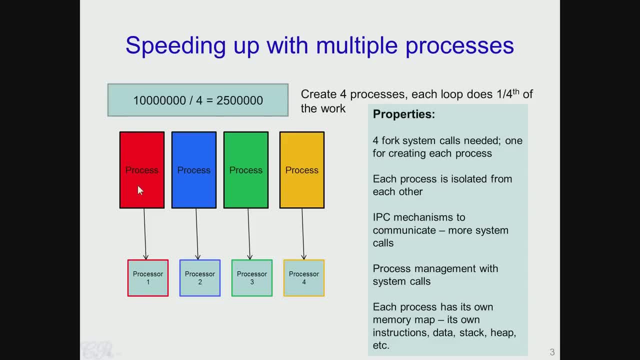 So every time one of these processes invokes a system call, it results in the operating system being executed, being triggered due to a software trap, and the operating system then determines what system call has invoked and the corresponding system call handler will be executed. So, as we have seen, 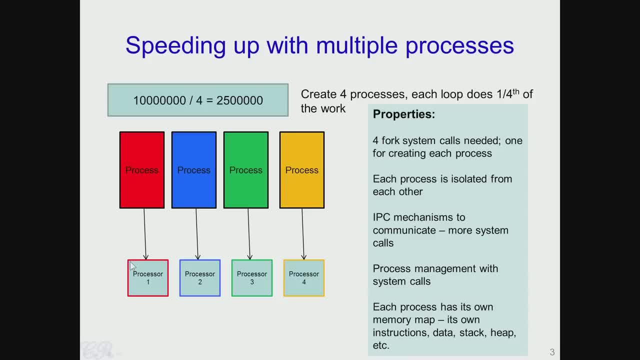 In an earlier video. this entire process could be quite considerable, And other overhead comes from the fact that a large portion of these four processes are similar. For example, all these four processes would have the same set of instructions which they operate upon and also they could be the same array which they are accessing, same global. 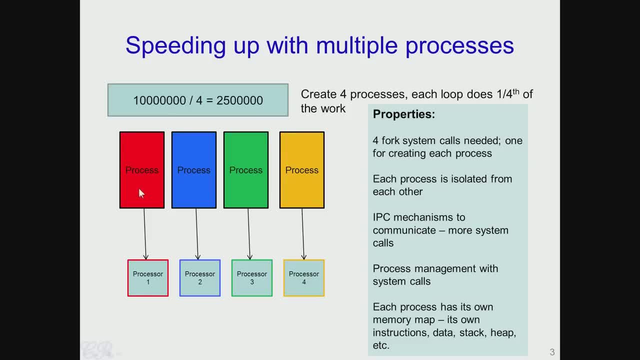 data which they are accessing And therefore, what we see is that there are 🔊🔊🔊 pieces of code often there we that there are a lot of duplication of instructions and data, which is happening due to having multiple processes which execute a job in parallel. 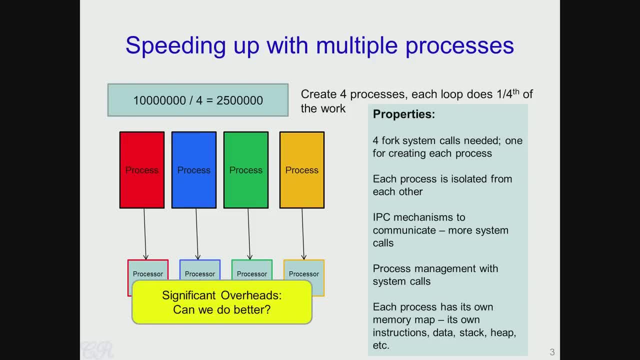 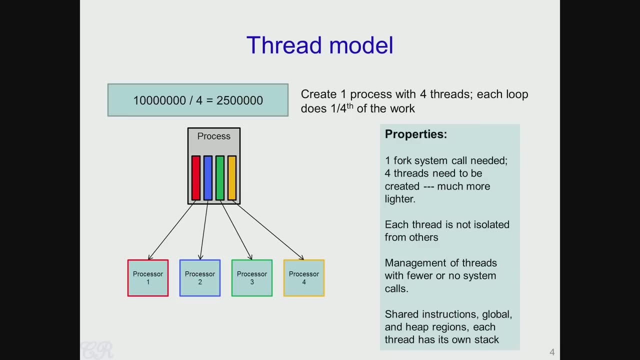 So is there a way we can do better than this? Is there a way we can have a solution where the amount of overheads present in parallelization can be reduced? So, in order to achieve this, what is used is the concept of threading. 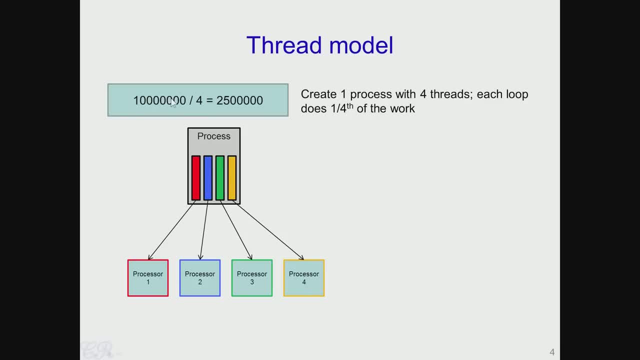 So, with threading, like before, we divide the entire space of 10 million into 4 parts of 2.5 million each, but instead of creating 4 processes, as we have done earlier, we will only create 1 process And within this process, we create a loop. 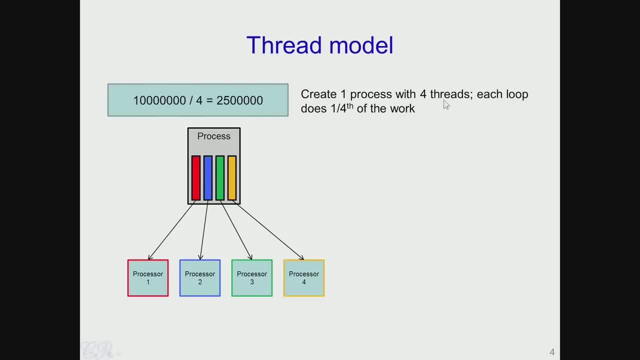 A execution entity which we call a thread. So each of these threads, quite like the previous idea where of using parallelized processes would have a loop which does a quarter of the work, that is, each of these threads, would find the sum of 2.5 million numbers. 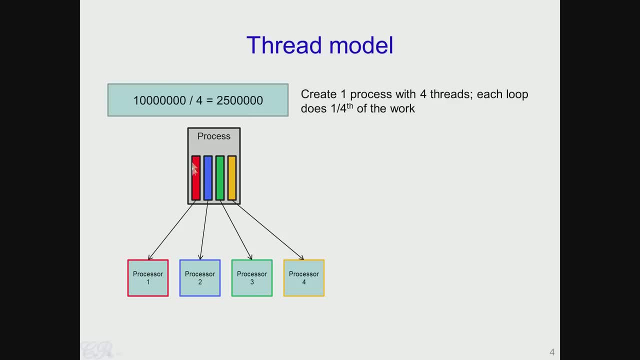 So, pictorially, this is what it is going to look like. So we have one process. So this one process would mean that it has one set of instructions, A global data heap and other segments and within this process, we have four executing. 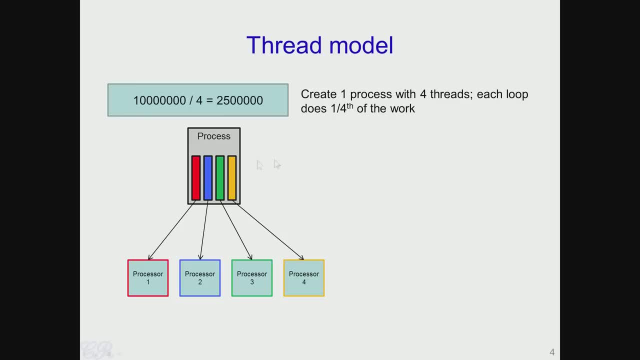 contexts. So these four executing contexts are the four threads and they execute within the particular process and each of these threads are executed in a different processor or typically executed in a different processor. For example, the red thread goes into processor 1 and is executing here. 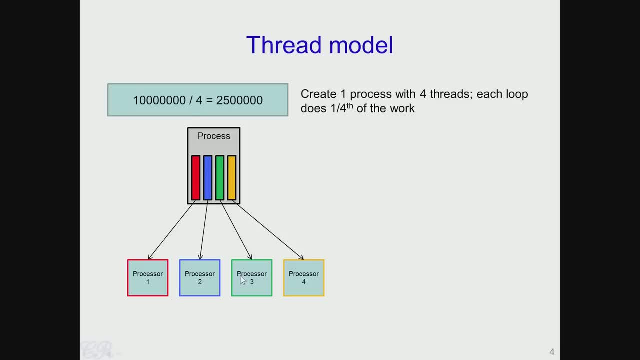 The blue thread goes into processor 2, green and yellow go into processor 3 and 4 respectively. Thus we are able to achieve parallelization by using threads. So this parallelization is quite similar, with respect to the process parallelization, what we seen in the previous slide. 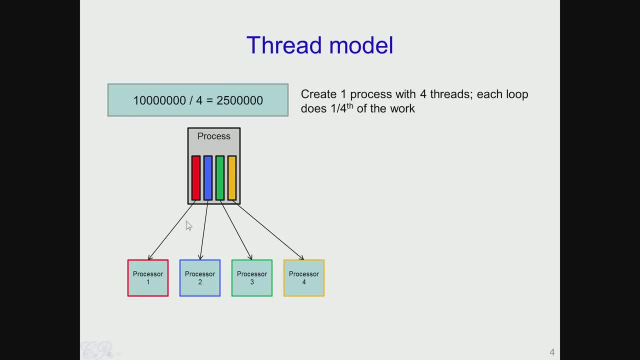 However, it has lower overheads. So the properties of this particular thread model of parallelization, So these two of a parallelization- is as follows: Since we have created only one process over here, so what we require is just one fork system call to create this process Now within this. 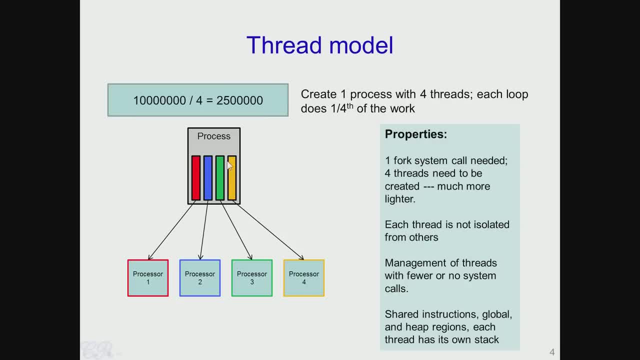 particular process. in order to create the 4 threads, we may use a library call, such as pthreadcreate, which may or may not require system calls. Further, a major difference with respect to the process parallelization from the previous slide is that these threads are not isolated from each other. So what this means is that 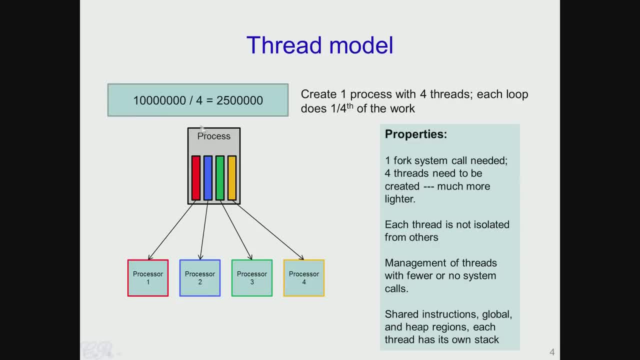 since all these 4 threads execute in the same process space, so these threads could access the process. So this process is segment, such as the heap segment and the global data. Also, it is possible that the instructions or the text segment in this process is also shared among the various 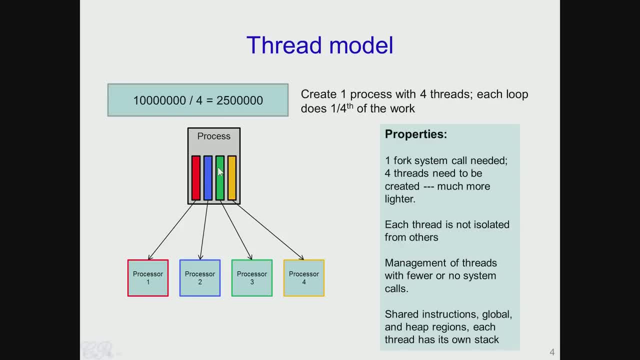 threads. Now, what is different, or what distinguishes the different threads, is that each of these threads will have its own stack, And having its own stack will allow it to have its own execution context. So each of these threads will be able to use the stack to create local variables, as well as to do 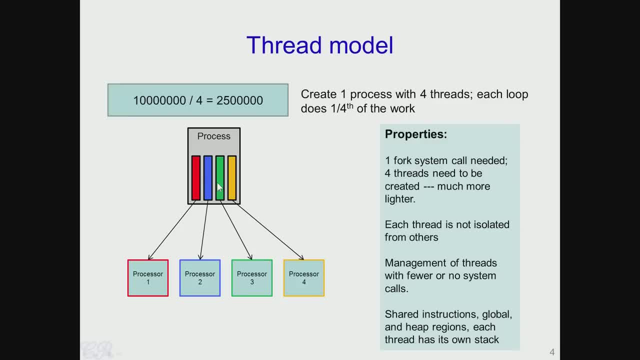 to store information about function calls and so on. Further management of these threads- that is, for example, waiting for another thread or exiting a thread- may not require to have system calls. So what we will do, So what we will see now, is these threads in more detail. So let us look at it with 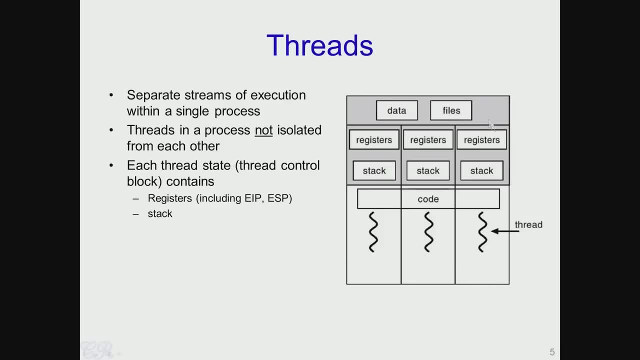 this particular figure. So we have this single process over here and within this particular process we have multiple threads. So these are the execution contexts of this process. So these execution contexts all share the same code and have access to the same global. 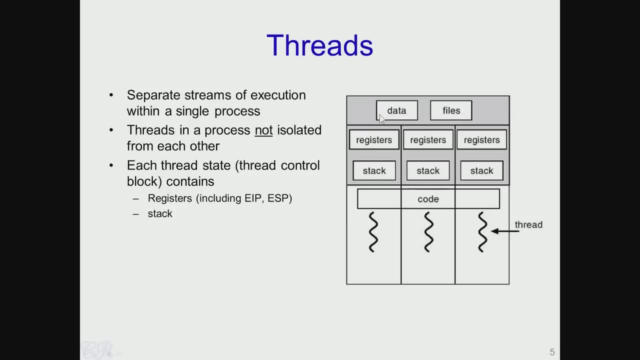 data And keep of the process, and also they will have access to the same files which are opened by the process. So what distinguishes one thread from the other is that each thread has its own stack which it uses for local variables and for function calls. 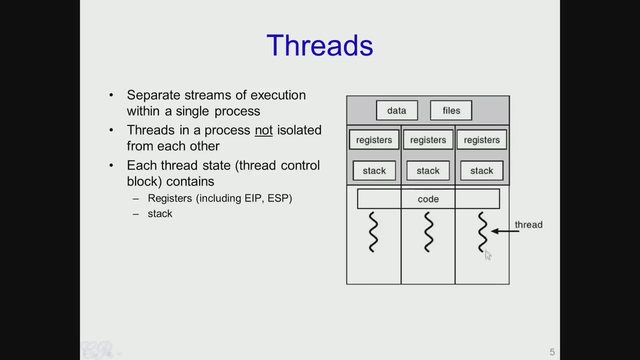 So these threads are, as mentioned, execution contexts, And each of these threads could be scheduled to run on one of the processors present in the system, or it could be also possible that these threads are scheduled on to the same processor, albeit at different time instance. Now, each thread is executing almost independently of each other. Therefore, 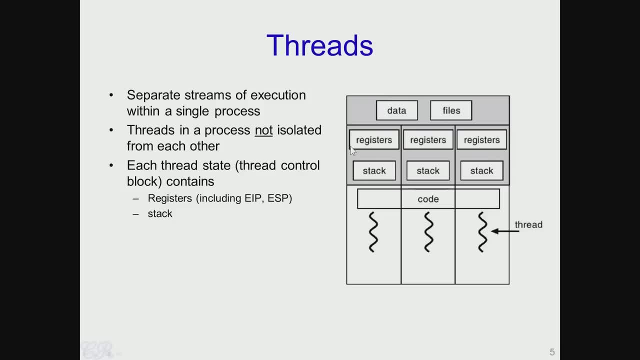 this registers over here signifies the execution context of a thread. So, as we have seen, each thread has its own execution context. So the execution context of this thread comprises of a set of registers like the EIP and the ESP register. Similarly, 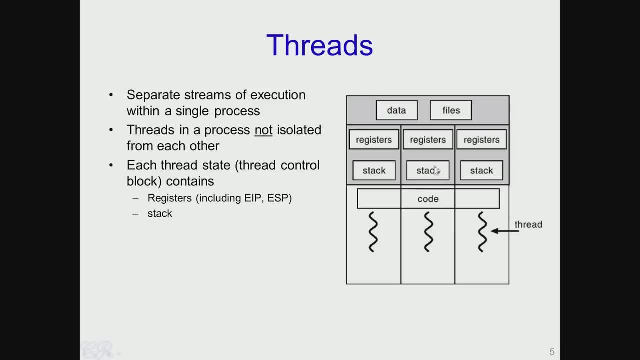 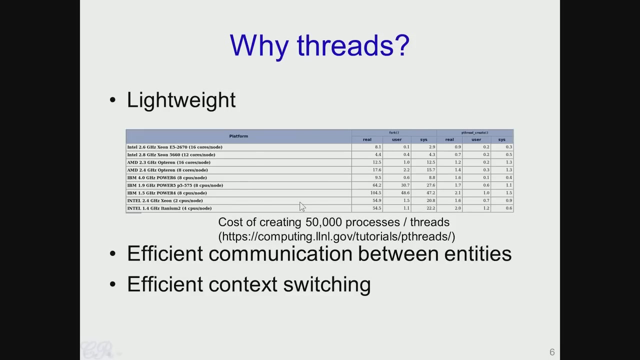 the execution context of this thread comprises of the stack and registers values. So these register values would help in the stopping and restarting of threads after or during a context switch. Now, what is the major advantage of having threads over processes? So this is actually seen from this particular slide. 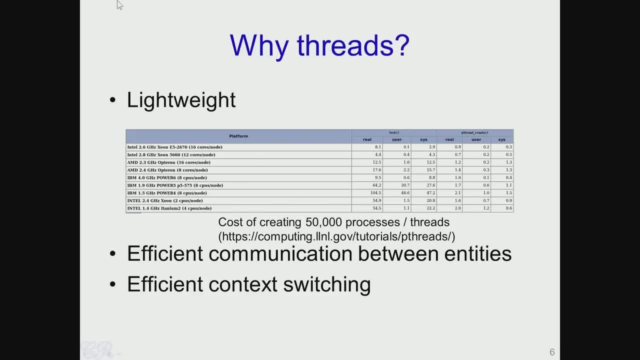 Essentially, the most important difference comes from the fact that threads are extremely lightweight compared to processes. To take an example, let us have a look at this particular table, which shows the time required to create 50,000 processes using the fork system call and it compares this: 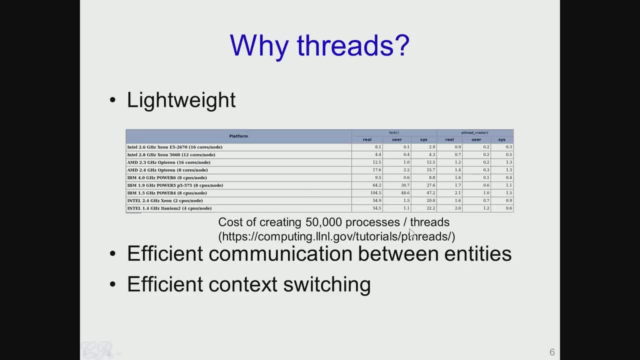 with creating 50,000 threads on exactly the same machines. So let us take any of these machines as an example. let us say the first one, and what we see- and if you look in this particular column which shows the time taken- is 8.1. 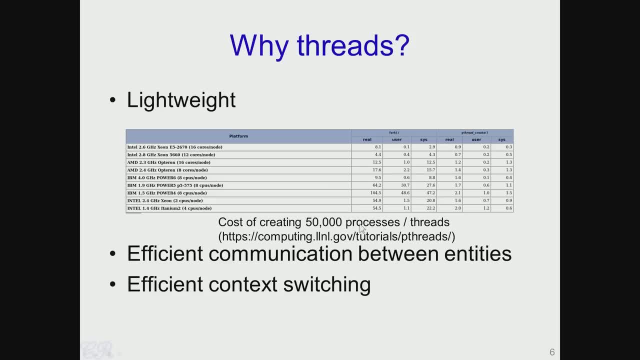 in order to create 50,000 processes using the fork system call. On the other hand, creating 50,000 threads on exactly the same machine only requires a time of 0.9.. So we see that creating threads are much more efficient than creating processes. 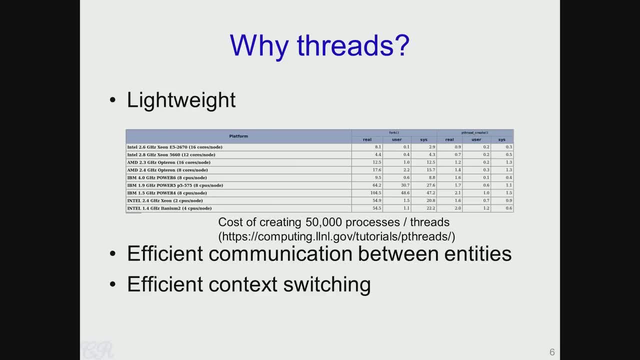 In a similar way. if we actually analyze other operations as well, We would understand that creating and managing threads are much more lighter than managing processes. Another important advantage of threads is that they are they allow efficient communication between the execution entities. For example, we have seen in processes, since each process is isolated from each other. 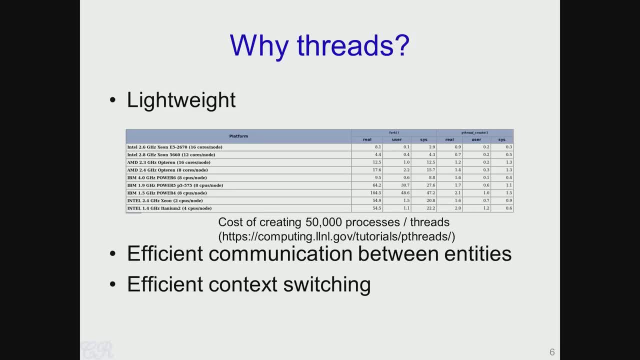 therefore, One way that processes can communicate is by IPCs and, as we have seen, IPCs involve quite a bit of system calls. So, for example, in the message passing IPC where we use send and receive, each send and receive invocation is a system call and has significant overheads. 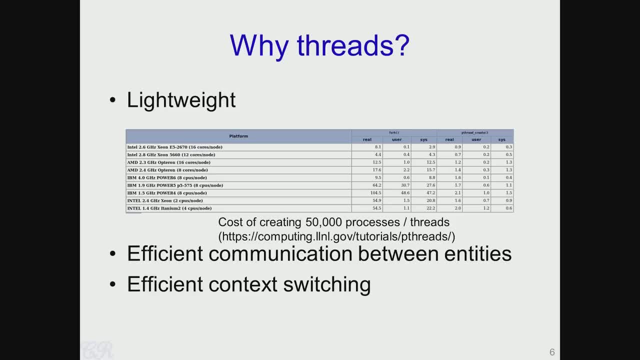 Similarly for shared memory IPCs. 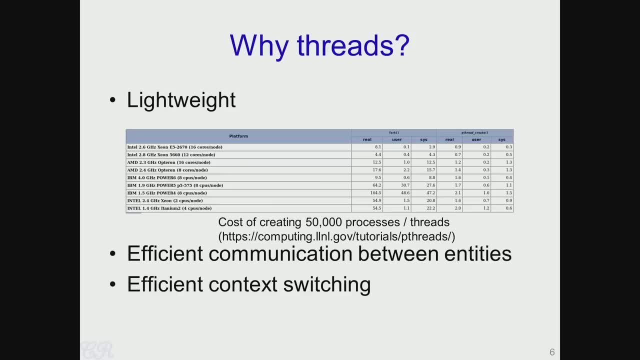 communication between threads in a single process can be easily achieved via the shared global data or, similarly, via the shared heap of the process. Another big advantage of threads is that it results in efficient context switching. So when we switch from one process to another, the context switching time is considerable. 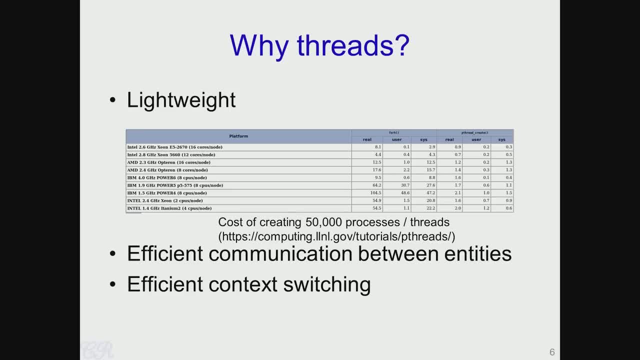 because the process state is quite large. Also, we require the TLB we flushed and the page tables for the new process to become active and this process, this new page table, would then be loaded into the TLB, and so on. On the other hand, switching from one thread to another first of all requires a smaller 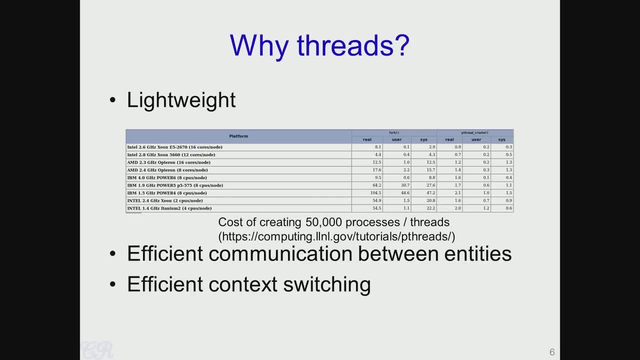 saving of the context, because the context of the thread is much more small. It is much smaller than that of a process. Therefore, lesser amount of context needs to be saved when switching between threads. Therefore, threads context switching would be faster. And other reason why context switching is faster in threads is that we are not changing. 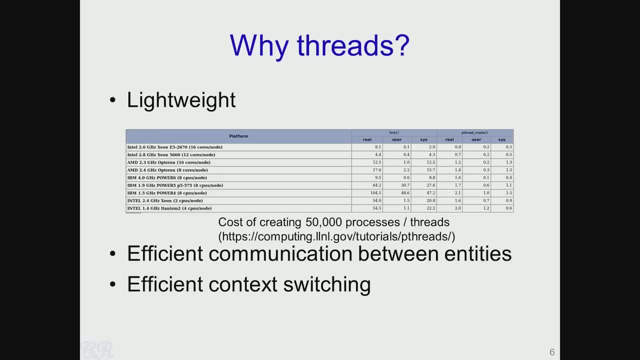 page tables. Essentially, since the threads execute from the same process and each process is associated with a set of page directory and page tables, when switching from one thread to another, this page tables and page directories will remain the same. Therefore, there is there are no overheads of making an other page table the active and 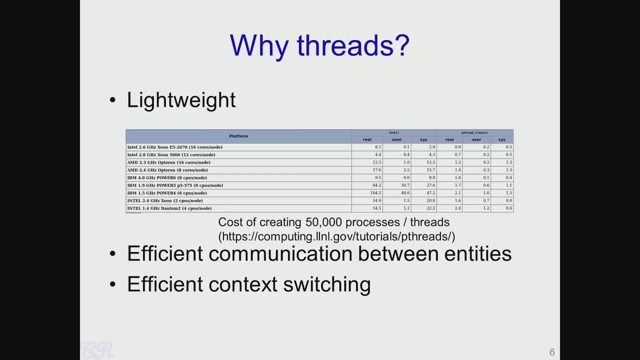 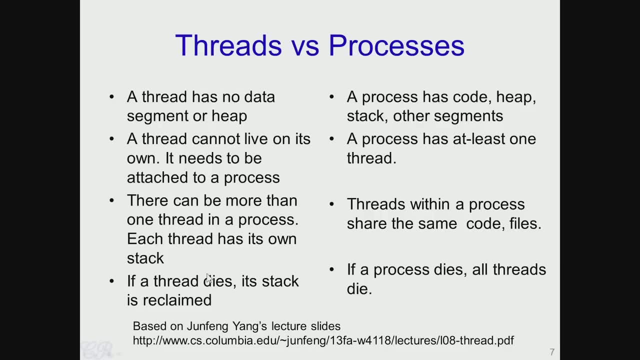 therefore, the locality is maintained and cached entries in the TLB will still be valid. So this particular slide reiterates a lot of differences between processes and threads, and we will quickly go through this. So essentially, a process is an isolated execution entity which has its own code heap stack. 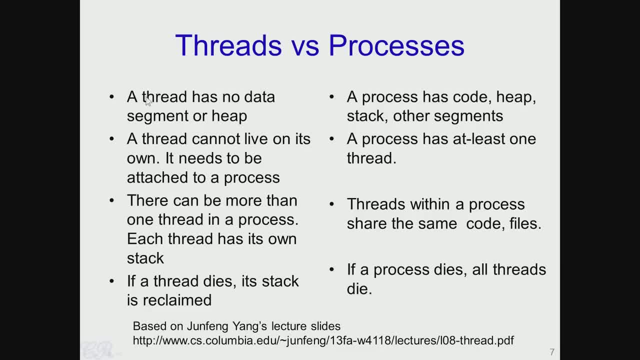 and other segments. On the other hand, a thread does not have its own data segment and heap and essentially it adopts or it uses the processes. So this particular slide reiterates a lot of differences between processes and threads- Though one and one are decision makers, have no объ excuse- which are just individually Datastick Team up, while context epicentrics that record the information then display them in the representation downtown which is some kind of consumer interface. So, this � ط kolay method can easily be uzi buy at z i. That is,aze to cooperate at different functions such as ujus, the w h o f the mapping. Causes data segment and heap. So all threads within a particular process would use the same data segment and heap. Another difference is that a process as itself is a complete entity, So a process you could consider it as having a single thread, that is, a single execution context. 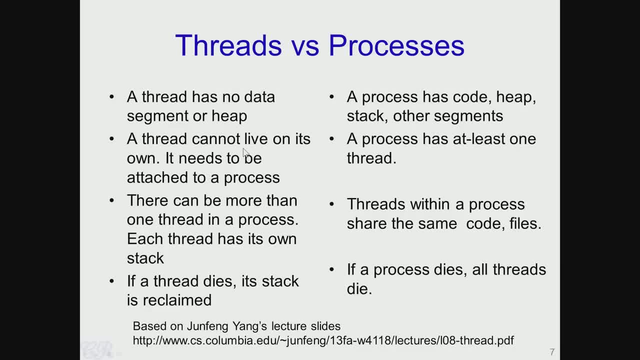 and could survive on its own. On the other hand, a thread should PCN on its own So can expect to compile some data so that the OK raw file could click in and said: good, 0 and 1.. a thread cannot live on its own, So it needs to be attached to a process. So when a process 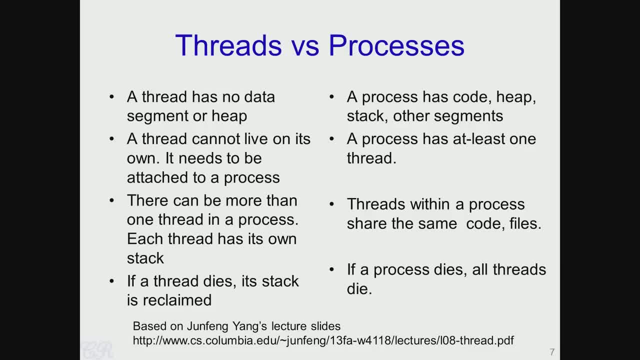 terminates, then all the threads that are present in that process will also terminate. So in other words, without a process, a thread cannot execute. On the other hand, a process would just have a single thread, and that is sufficient for the process to execute. So why do we say a single? 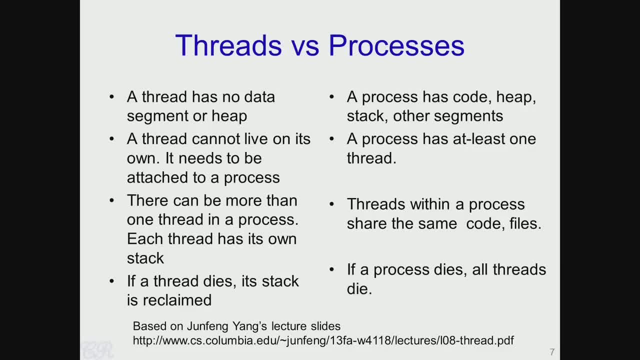 thread. This means any execution context of a process forms the single thread. So threads within a process share the same code and files, as we have seen in the earlier slide. But each thread has its own stack and this stack is reclaimed when the thread dies. So it is possible that. 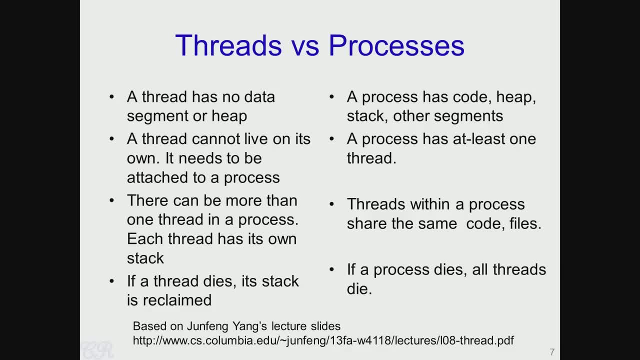 I. So when a thread terminates, the remaining of the process will continue to execute. For example, if a process has, say, 10 threads and one of the threads terminates, then the remaining 9 threads will continue to execute. On the other hand, if a process terminates, then all threads within that process will. 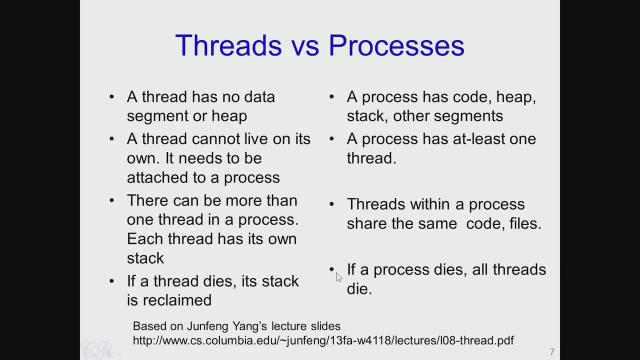 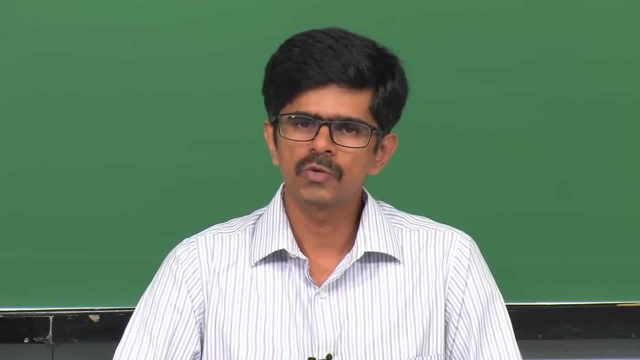 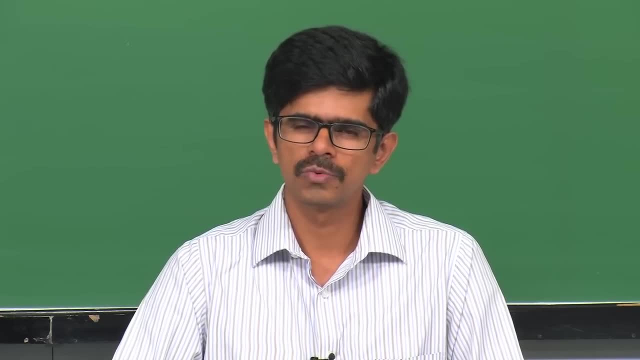 also die or will also terminate. So how do we create and manage threads? Now? there are several libraries to do so, but what we will look in this particular video is a very popular library known as the Pthread library. So we will see some of the very critical or very important functions in the Pthread. 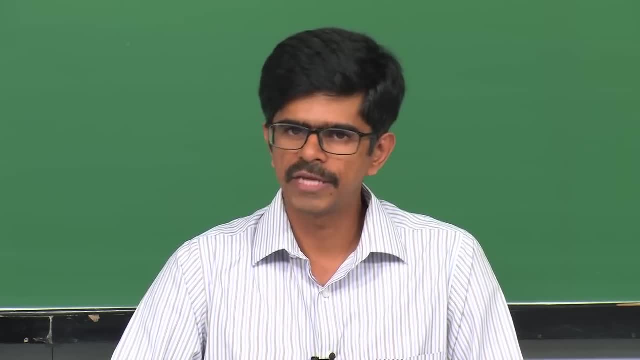 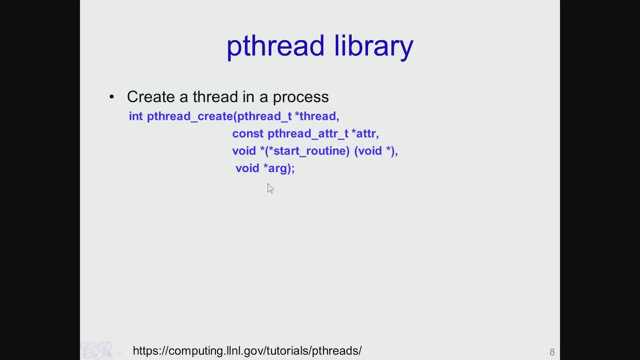 library which are used to create and manage threads. So let us see how we could create a thread in a process. So, in the pre, So in the Pthread library, a thread is created by using this function, pthread create, which takes several arguments. 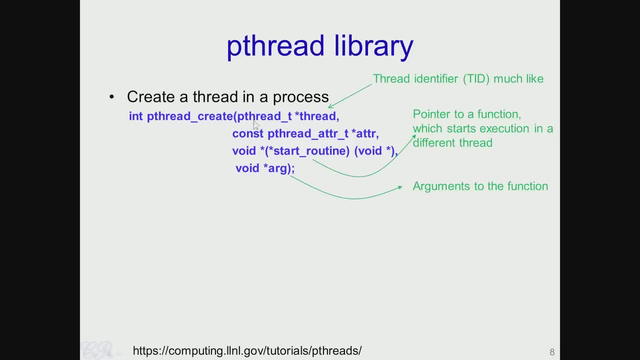 So it takes like four arguments and these four arguments are as shown over here. So the first argument, which is of defined of form, which is a pointer to pthread, underscore t is the thread identifier or tid. So this is very similar to the process identifier or pid, which we have studied in the previous. 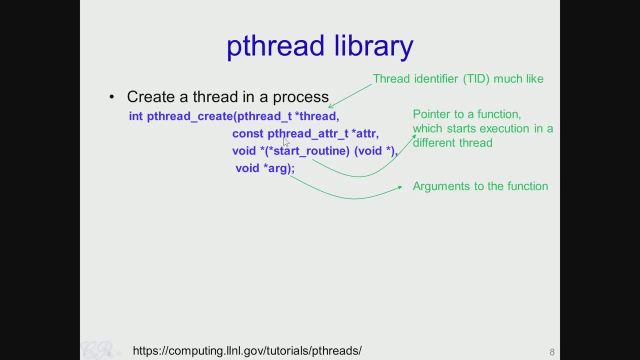 video. The second argument to pthread create is the attribute. So through this attribute you could specify several properties of the thread that you have been creating. So what pthread would underscore create function would do is that when it is invoked, it is going to create a thread context, or rather a new thread context in the process, and it 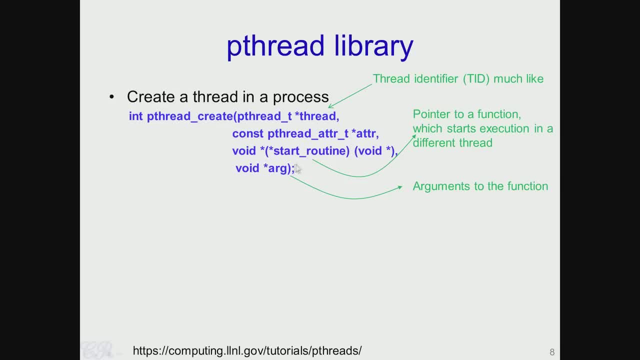 is going to start executing that new context context from this function specified over here. So this third parameter specified as start underscore routine is a pointer to a function which begins to execute in the new thread context. So this function will start to execute in a different thread. 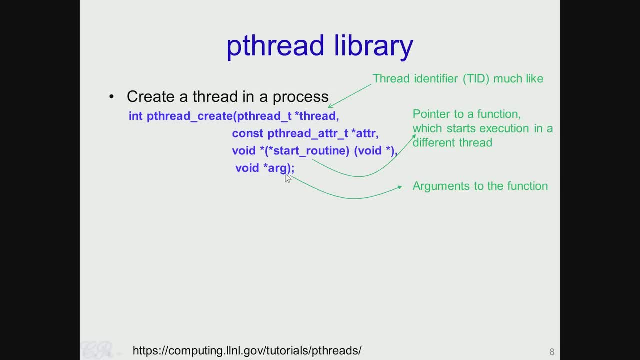 The last argument for pthread create is arg or arg, which is a pointer to the arguments to this particular start routine function. So in the next couple of slides we will see examples of how to use pthread create and also examples of the other functions in pthread. 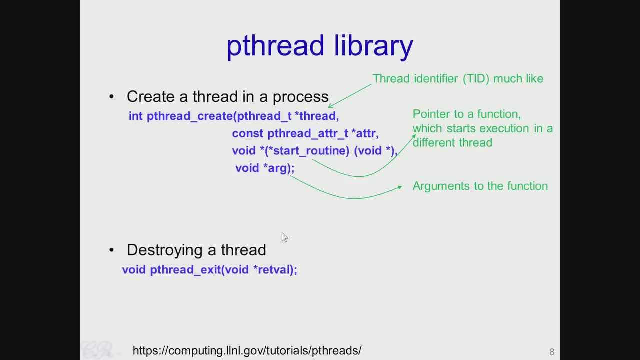 So now that we have created a pthread and let us say it has done its job, the next thing is to actually destroy a thread, and this is done by this function called pthread underscore exit. So pthread underscore exit will also pass the pointer to the argument. 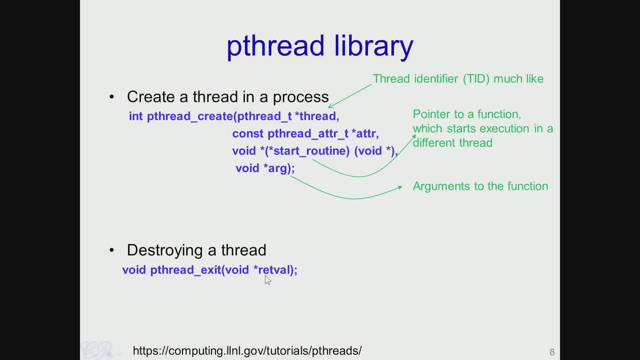 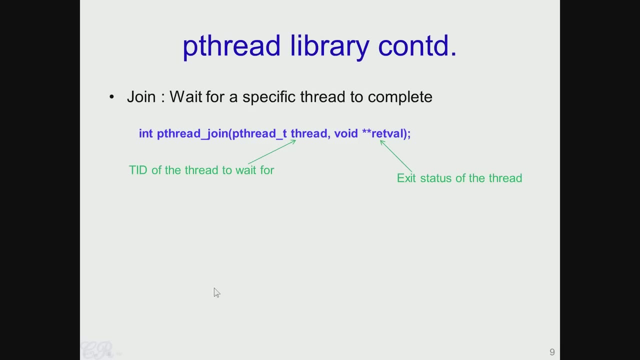 The return value in order to pass the return status of the thread. So this is in many ways similar to the exit system call that we have seen in processes. Now, another important pthread library function is this particular function called pthread underscore join. So 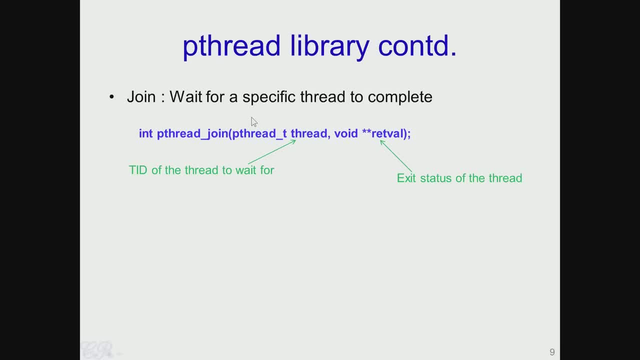 through this, a process or a thread could wait for a specific thread to complete. So this is much like the wait system call that we have seen with respect to processes. So in pthread underscore join, what is specified is the tid of the thread to wait for. that is the thread id of the thread. 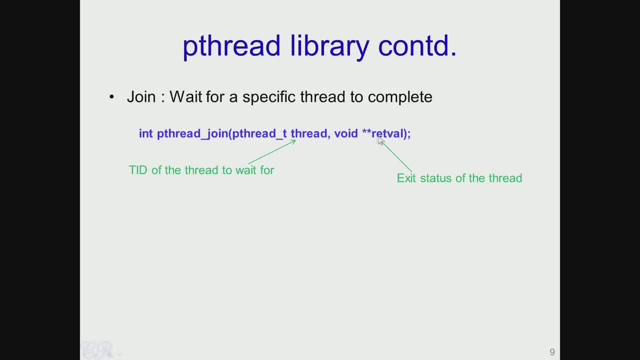 and what is obtained over here is the exit status of the thread. So this pthread underscore join will block the calling thread until the thread specified by this tid passed over here exits. and when the thread exits, then pthread underscore join will wake up and it will be able to. 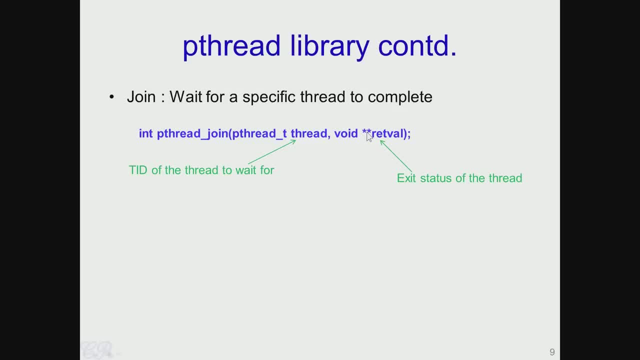 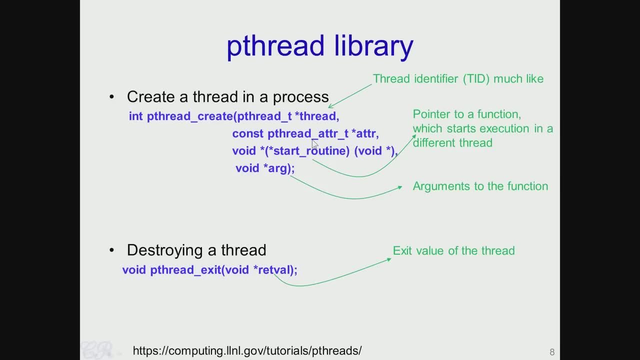 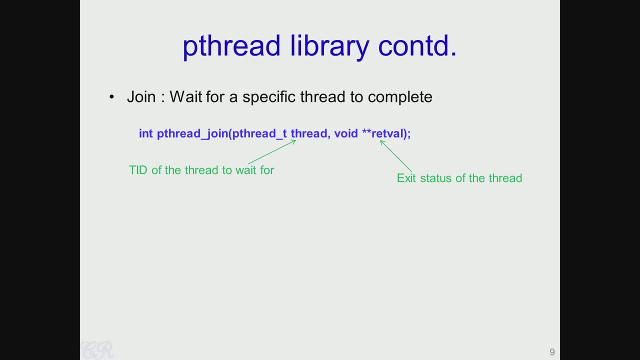 read the exit status of the exited thread specified by the TID. So, given these particular three functions- pthread underscore create, pthread underscore exit and pthread underscore join- Let us see how we could use these pthreads in order to parallelize our program of finding. 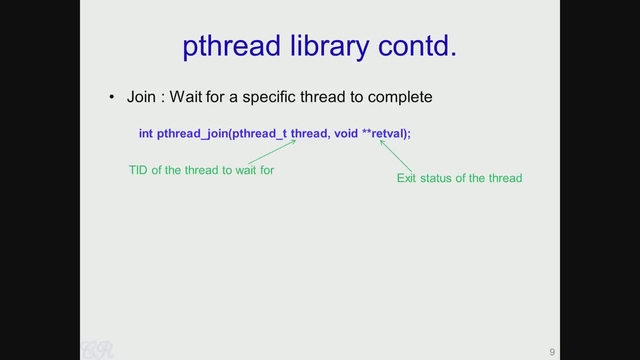 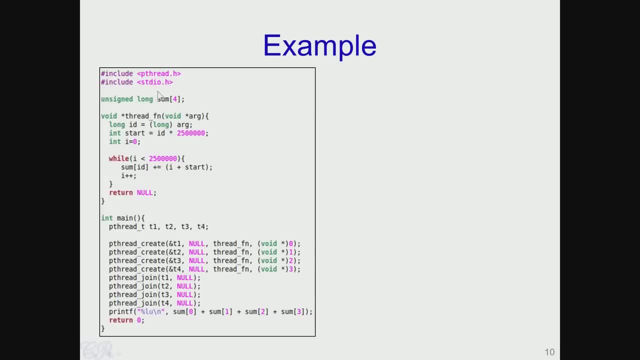 the sum of the first 10 million positive integers. So this is the code to do that. So what this particular code does is that it creates 4 threads and each thread finds the sum of a different 2.5 million. 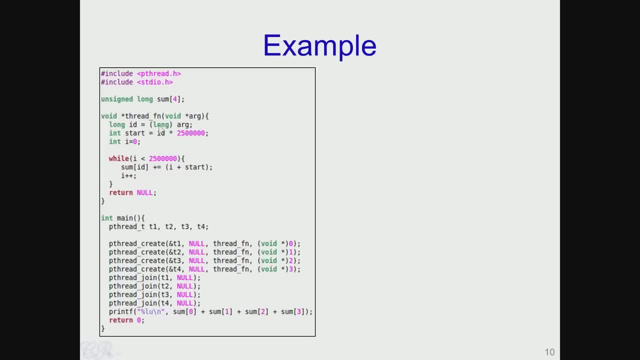 set of numbers and these 4 threads execute in parallel and therefore very quickly find the different 2.5 million numbers, and then we add the results to get the sum of the first 10 million numbers. So let us see this example in more detail. 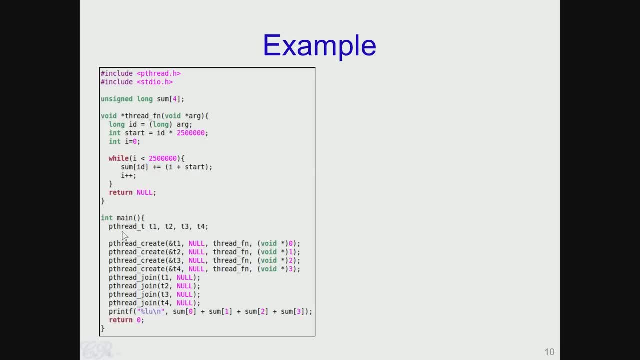 So, first of all, we defined 4 variables of type P, thread underscore t. So these are the t 1, t 2, t 3 and t 4.. So these are going to be used to create the 4 threads and these 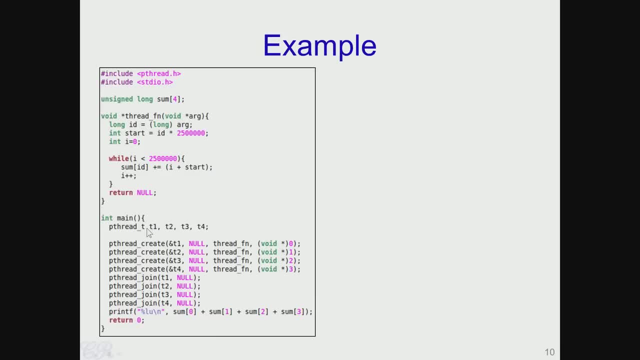 specific would contain the. So these are going to be used to create the 4 threads, and these specific would contain the thread ID or the TIDs. Now, as we have seen in the earlier slide, creating the thread is done by this function called pthread underscore create. So each of these pthread underscore. 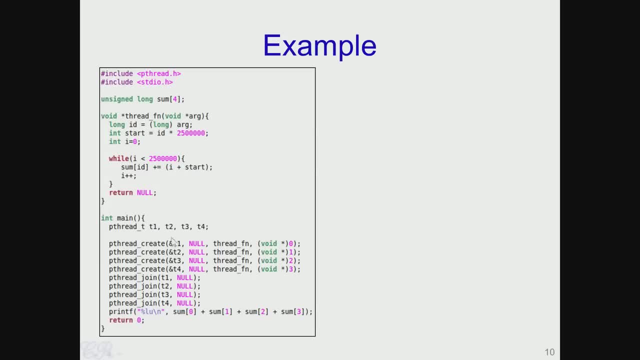 create invocations would pass the pointer to one of this, that is, T1,, T2, T3 and T4, which then gets filled with the thread identifier or the TID of the newly created thread. The second parameter, that is, the attributes of the thread, is specified as null, while the 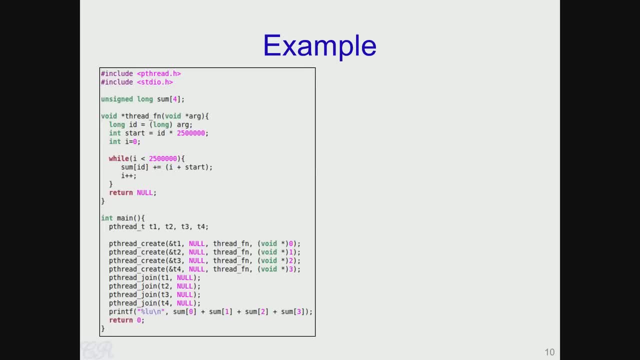 third parameter is function pointer, which specifies the function where the thread should execute. So over here the function pointer is a pointer to this function, thread underscore fn, which is defined over here, and it takes an argument void star. that is specified over here, arg. So the last parameter which is passed to pthread. 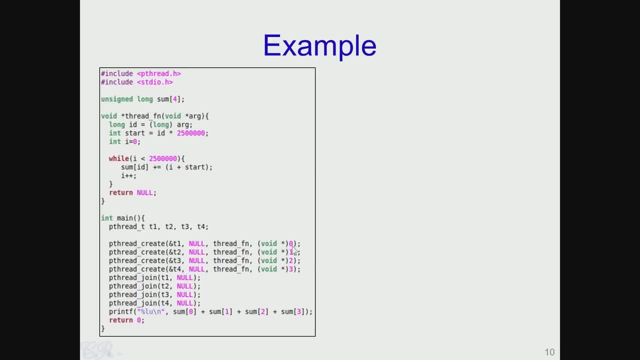 underscore create is the argument which would be passed over here in the arg of this particular function. So in this way, when pthread underscore create is invoked, it would create a thread context in the process and this thread context or this execution context will begin to execute. 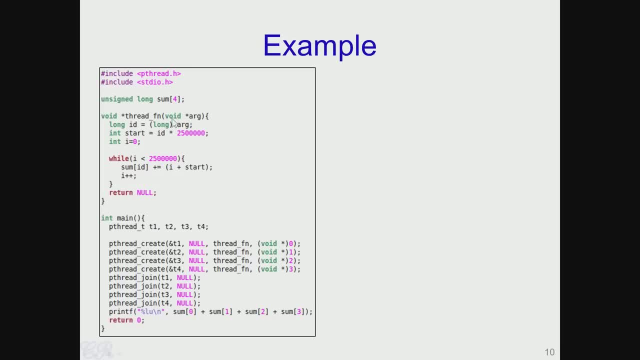 from this particular function. Now the argument passed in this particular thread would be as specified in the last argument of pthread. In this way we have invoked 4. pthread underscore creates and thus creating 4 threads within the single process. All these 4 threads have the same starting function, that is, thread. 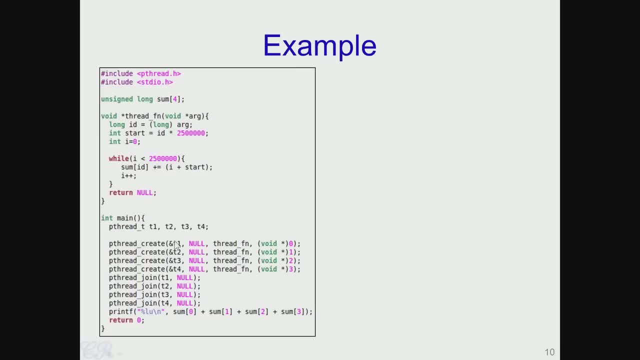 underscore fn and the thread ids will be filled into this first parameter, that is, T1, T2, T3 and T4 respectively. Now, each of these 4 threads which will begin executing from this thread function, which is, like you could think of, like the main of 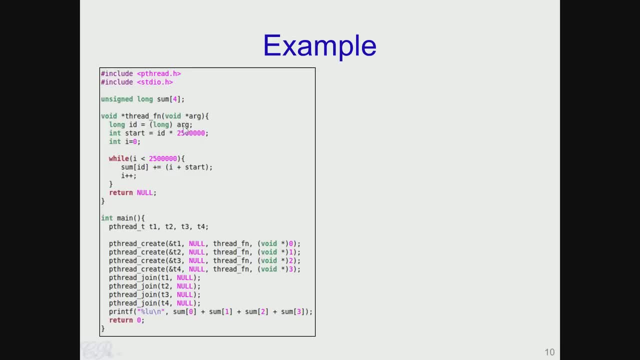 the thread would see a different value of arg. For example, thread 1 would have a arg value of 0, thread 2 would have a arg value of 1, thread 3 would have an arg value of 2 and thread 4 will would have an arg value of 3.. 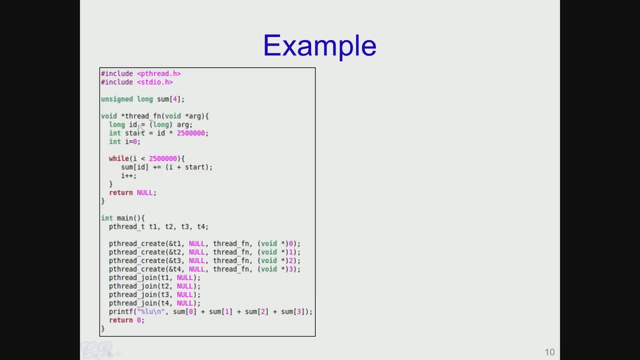 So using this arg value, which is then type casted to ID and then it is actually used to determine the start. So start is then used to determine which of the 2.5 million numbers the particular thread should add, For instance, if the arg past arg inner thread. 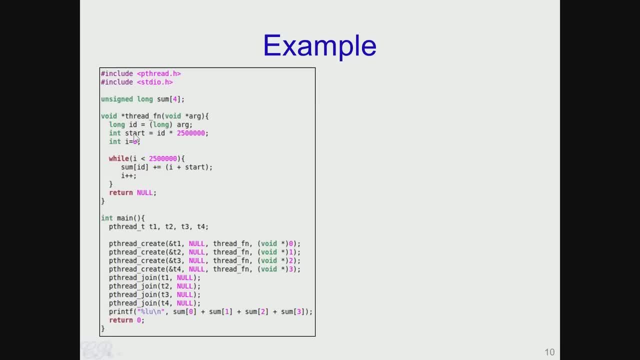 is 0, then the value of id of typecasting is 0 and the start value would also be 0. So this thread with the id 0 would add the first 2.5 million numbers, that is, the numbers from 0 to 2.5 million. 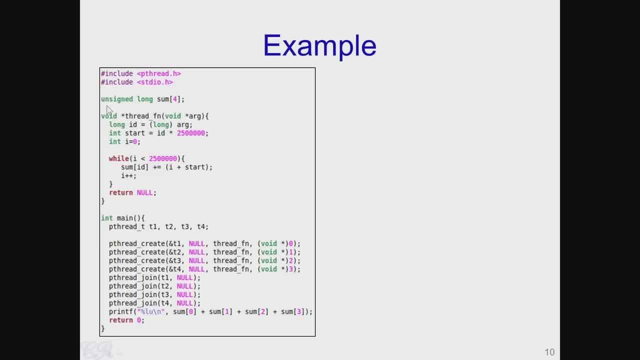 Now, in addition to this, what is defined is a global array called sum. So this is unsigned long array of 4 elements. Now this sum is used to accumulate the sum for each thread. So sum 0 would contain the sum of the numbers from 0 to 2.5 million, which is filled by the 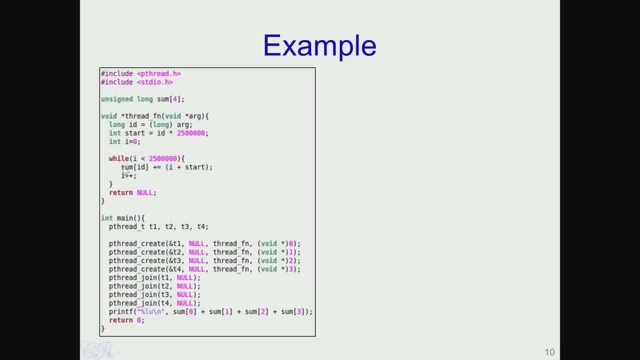 thread 0.. Ok, Or thread 1, that is the T1 thread. Similarly, sum 1 will have the sum of the numbers from 2.5 million to 5 million, and this sum of 1 is filled by thread T2.. In similar way, sum. 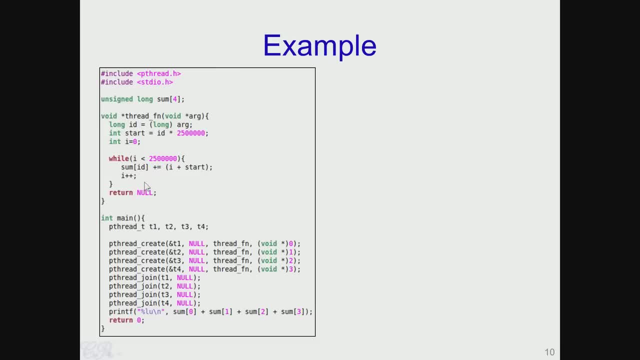 2 and sum 3 would have the corresponding 2.5 million sum and it is filled by T3 and T4.. So while this process is going on in the 4 threads- that is, the while loop, which takes considerably long time- is being executed by the 4 threads independently. What the main thread does is. 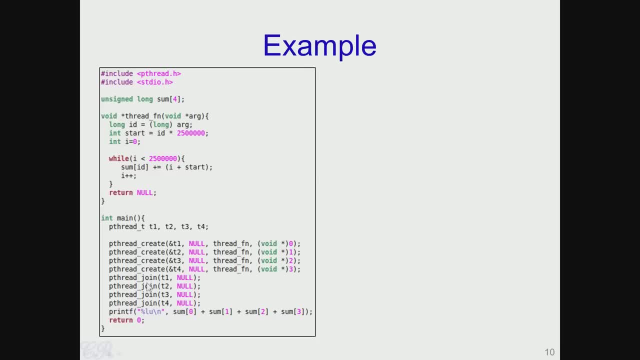 after creating the 4 threads, it will invoke join. So it invokes 4 joins corresponding to the 4 threads, and what this join call would do is that it is going to block until the corresponding thread specified by the TID. Ok, So the TID over here will exit. Thus, when thread T1 exits from this particular function, 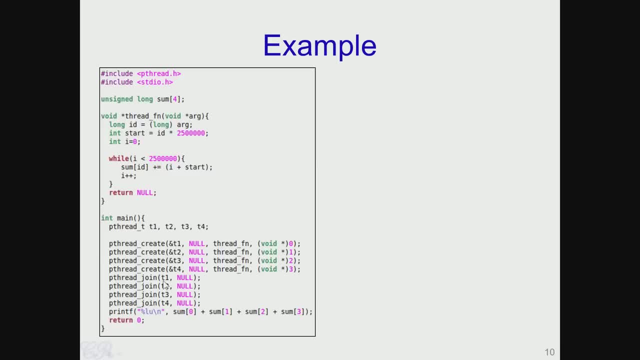 this pthread underscore join of T1 will wake up and it will complete executing. So in this way, all 4 join functions, on completing, will indicate that all the 4 threads have completed their execution. Then, after the 4 threads have exited, the 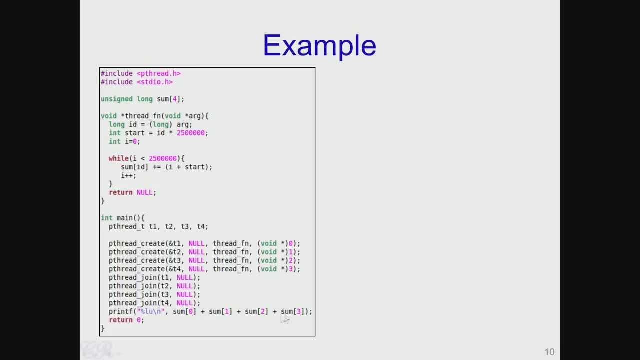 elements of sum which contain the partial sums of the 2.5 million numbers, are taken and added to get the final result which is printed on to the using the printf. So this final sum printed is the sum of the first 10 million numbers and therefore we have seen that the large job 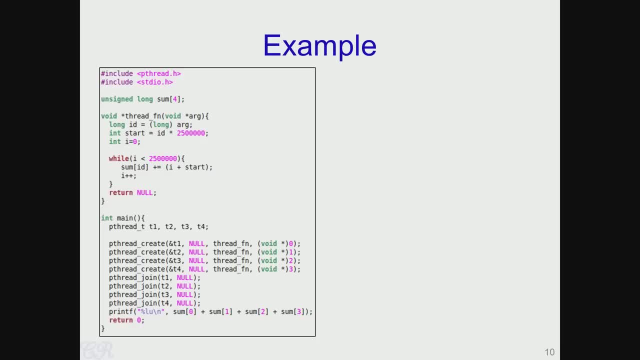 of adding numbers from 0 to 10 million is broken down into 4 parts, and each part is then cut. work is then computed by a thread to get a partial result which is then added on. Now, in order to execute and run this program, we use something like gcc thread dot c, which 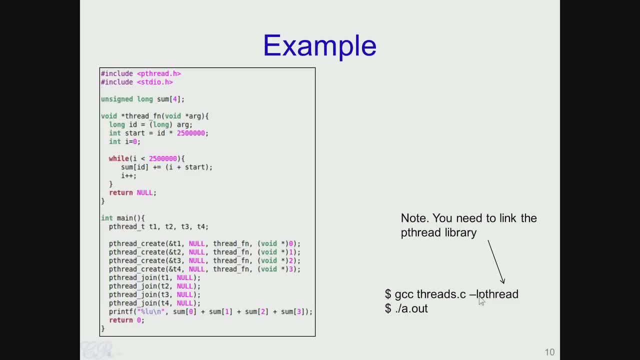 is the compilation, and we also specify a minus lp thread, which is the pthread library, which also needs to be linked into this particular executable. So gcc would result in an a dot out executable which is then going to be executed. So you can actually try out this particular program on a Linux system and you could try. 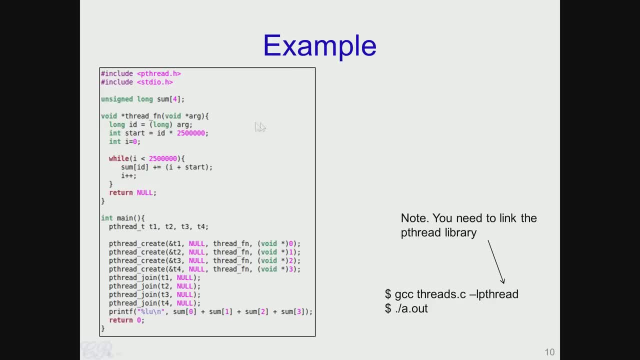 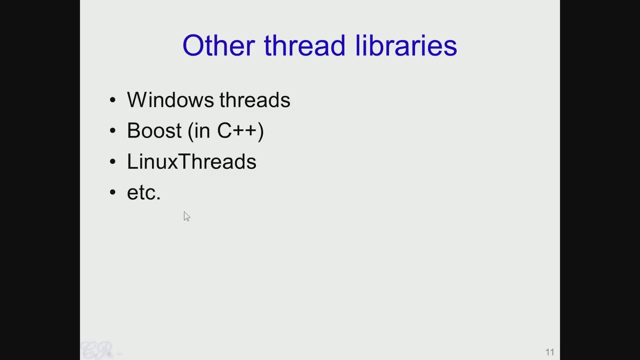 to determine the amount of speedup that you obtain by having a different threads to do the job compared to different processes, and also a sequential program where you have only one process executing this job. Besides the pthreads, there are several other libraries which you could possibly use to